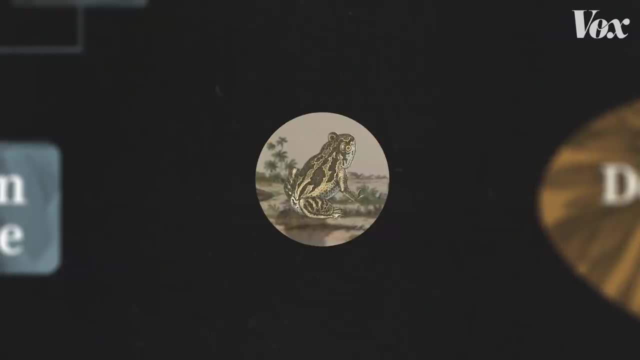 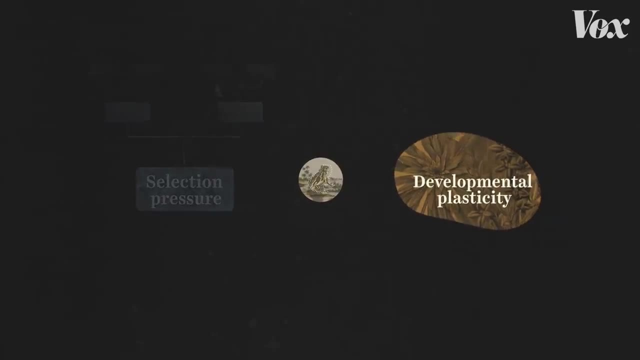 It's the same idea, But cold-blooded animals don't generate body heat, and they're shrinking too, which means that selection pressure for conserving body heat isn't the only thing at play. Instead, cold-blooded animals are particularly susceptible to plastic changes. 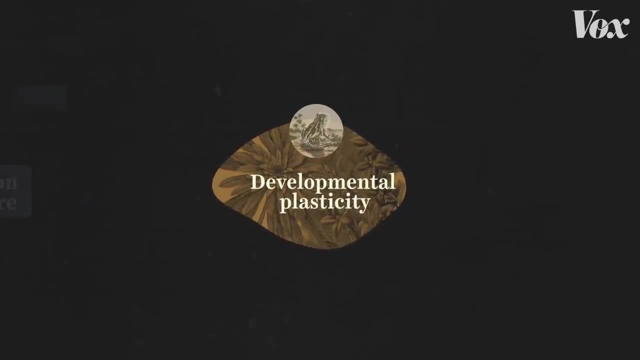 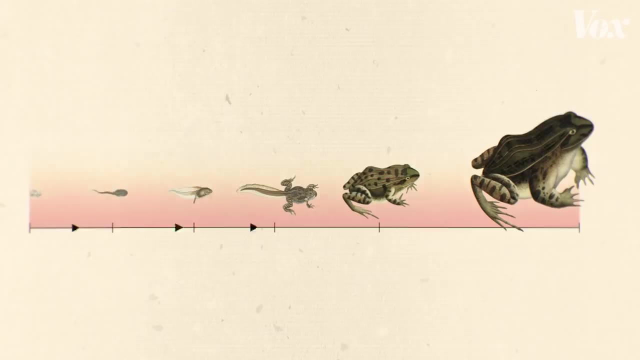 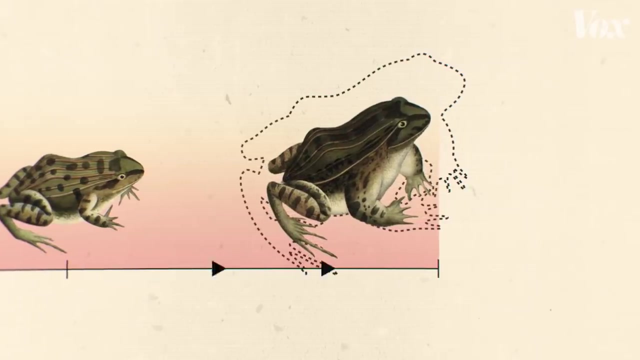 Changes that occur during the individual's lifetime and aren't passed on to the next generation. With frogs, for example, warmer temperatures increase metabolism and make the transitions between lifecycle development phases speed up, But because their rate of growth doesn't change, they're smaller by the time they arrive at adulthood. 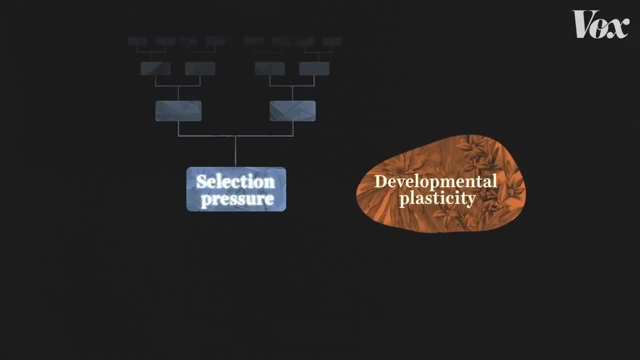 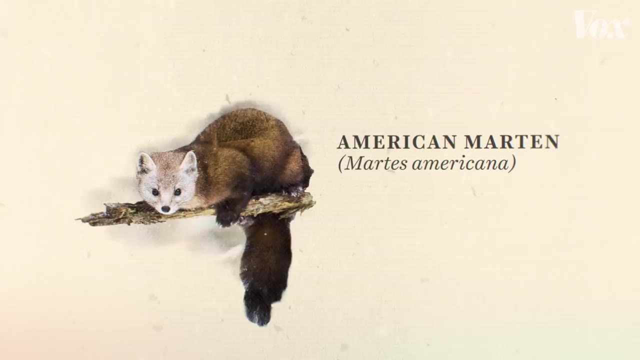 What researchers are still trying to figure out is how much these two factors are shaping warm and cold-blooded species and whether they can make predictions about what those changes will look like. Plus, this trend isn't uniform: Warming temperatures are making some species bigger. 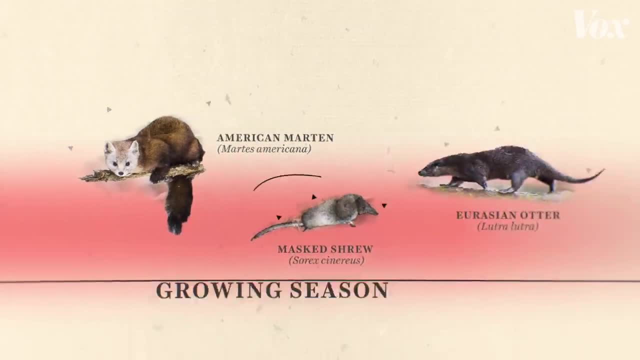 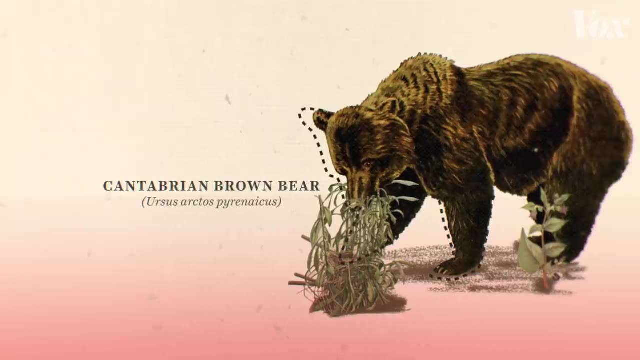 In high latitudes. increasing temperatures and precipitation have given shrews, otters and martens more time and resources to grow before winter. But we do know that warming results in smaller animals on average, because Earth has been through periods of warming that have shrunk animal bodies before. 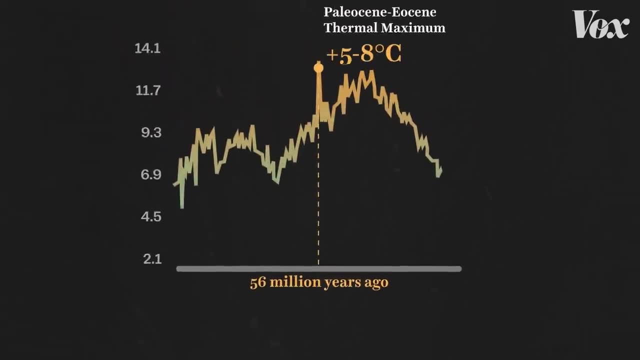 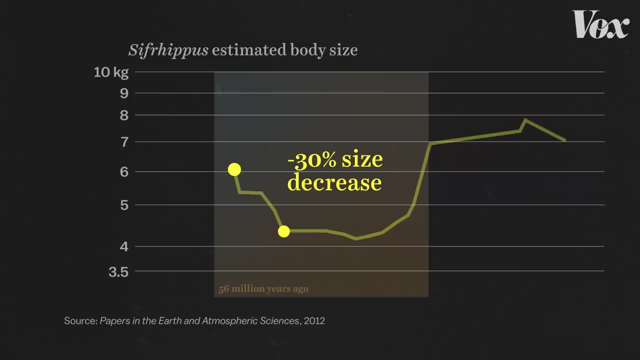 In a warming event roughly 56 million years ago. temperatures increased between 5 to 8 degrees Celsius over 10,000 years And we can see a noticeable dip in animal size in the fossil record. But today we're warming the planet at an unprecedented rate. 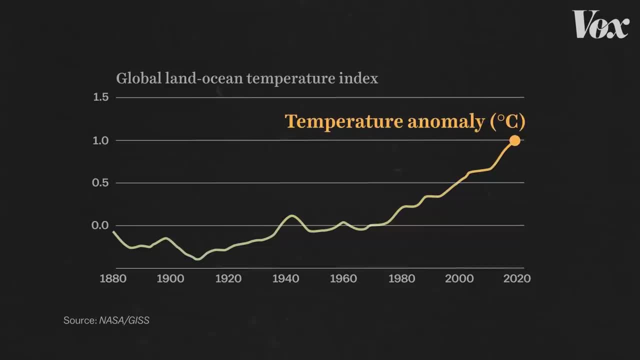 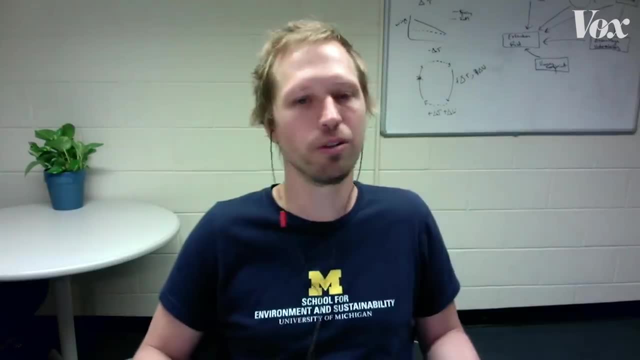 about 10 times faster than the average warming following historic ice ages, giving animals little time to adapt. That's the problem with human-driven climate change. It's the rate of change that's just orders of magnitude faster than what the natural world has had to deal with in the past. 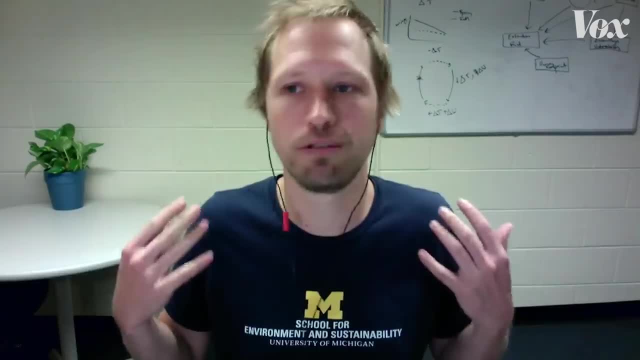 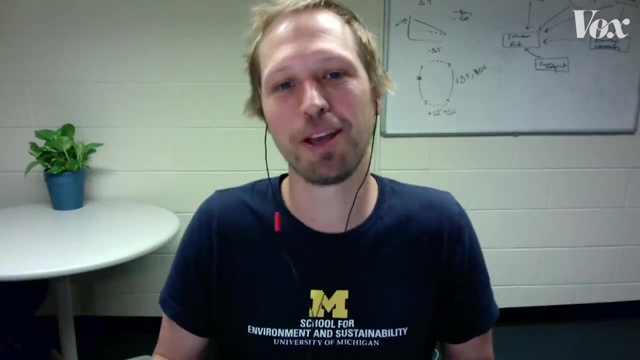 Size is really important to think of survival, and you can't just change that indefinitely without consequence. For one thing, I don't think it's feasible that species are going to be able to continue to get smaller and maintain things like a migration from one hemisphere to another. 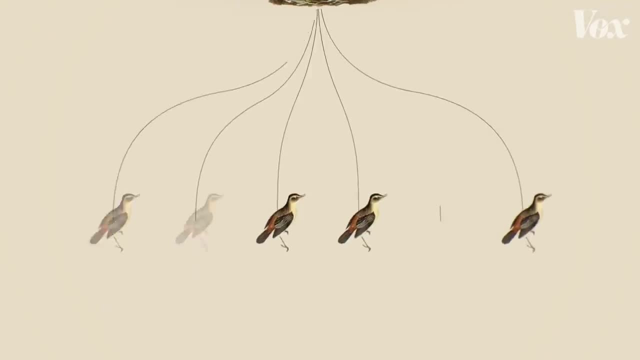 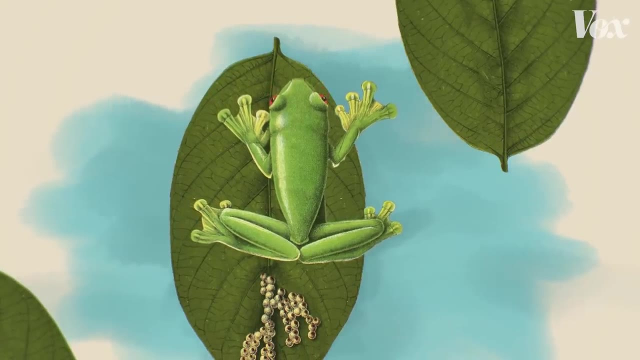 And since smaller bodies can hold fewer eggs, they result in fewer offspring and a lower population size in the long run. For amphibians, who need to keep their skin wet in order to breathe, shrinking can mean higher chances of drying out in a drought.